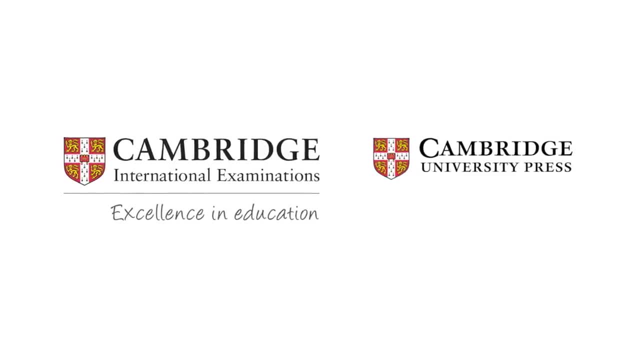 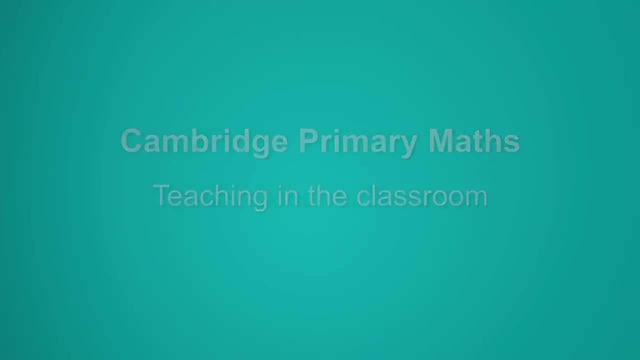 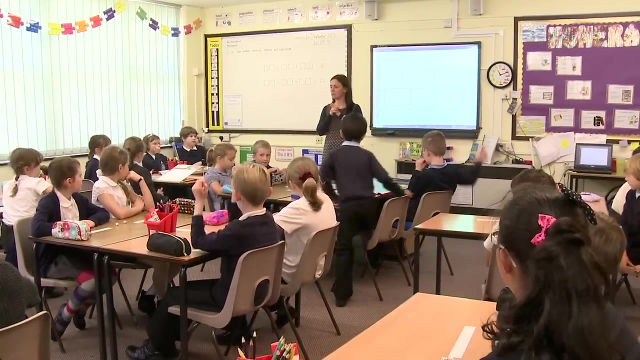 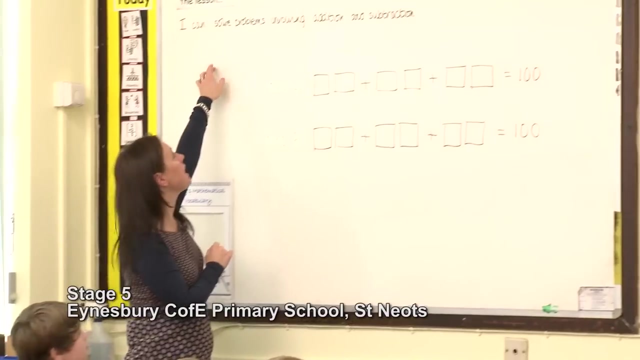 At Ainsbury C of E Primary School in St Neots, a Stage 5 Maths lesson is starting. So what we're going to do to warm ourselves up today- Year 5, is we're going to be playing a game. Today's lesson is all about problem solving with addition and subtraction. 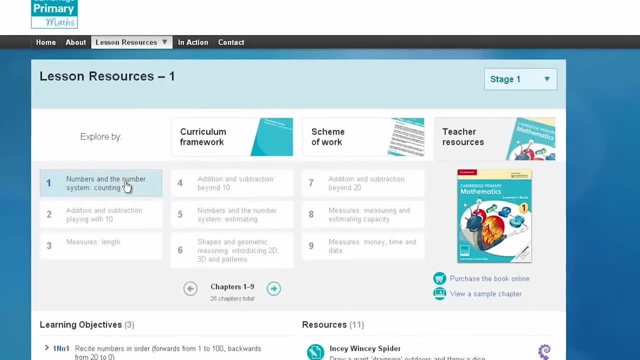 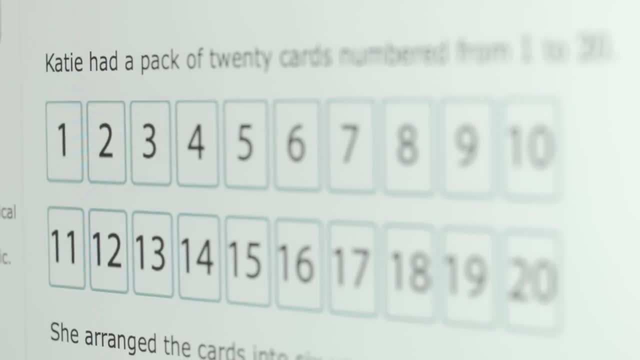 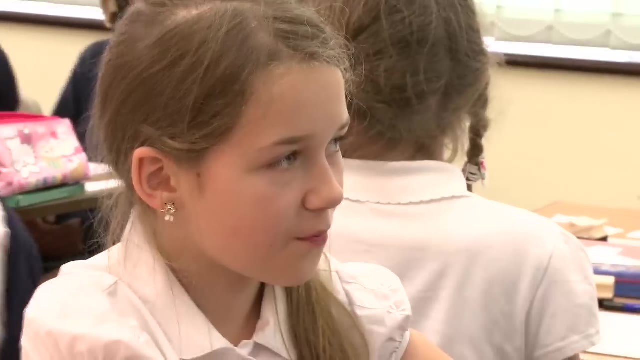 The teacher uses an activity from Enrich 20 divided into 6, to introduce learners to the idea of problem solving in mathematics. The aim of the activity is to create six piles from 20 cards. Each pile has to add up to the same total. 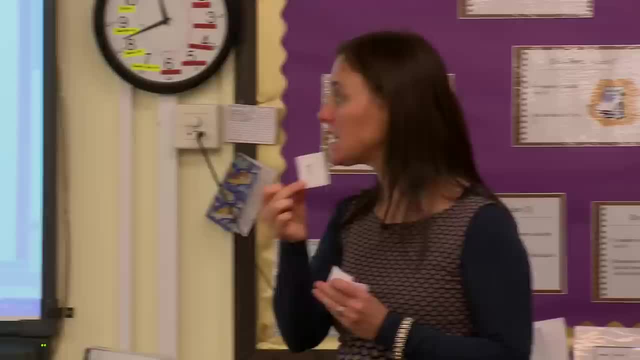 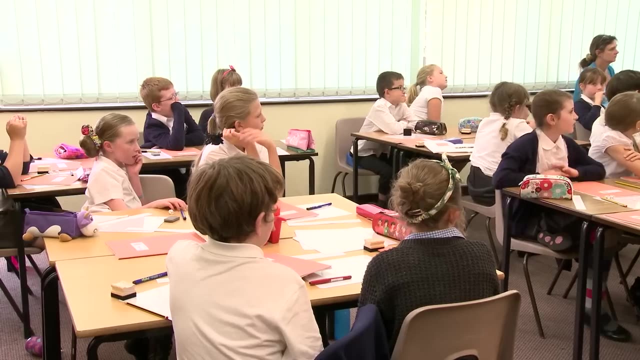 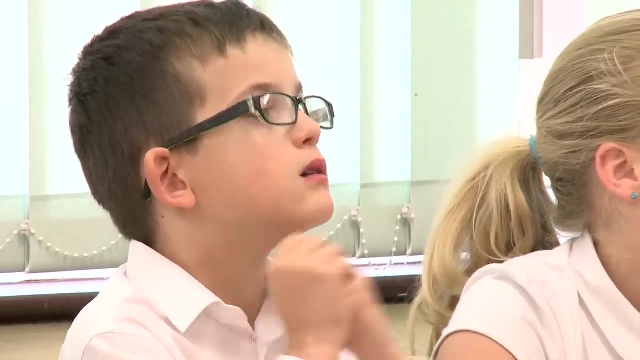 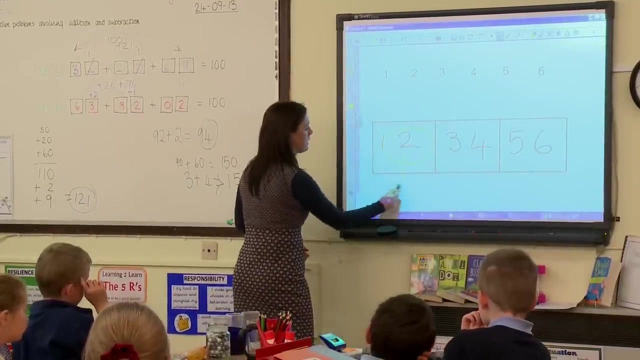 Organise these into six piles so that the total in each pile is the same. To start with, the teacher simplifies the activity. She demonstrates an easier version by creating only three piles from six cards. One add two is three. This is really easy math. One add two is three, Three add four. 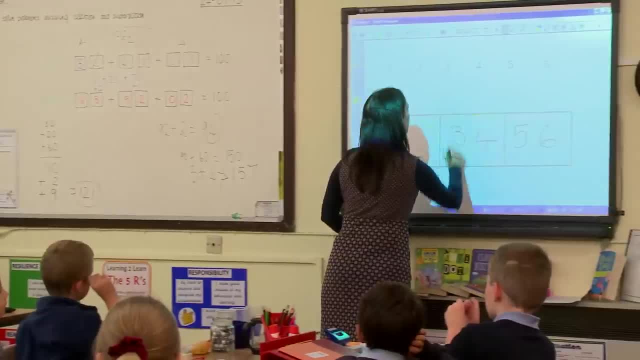 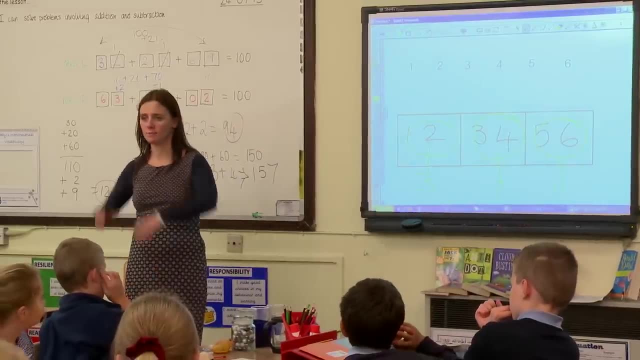 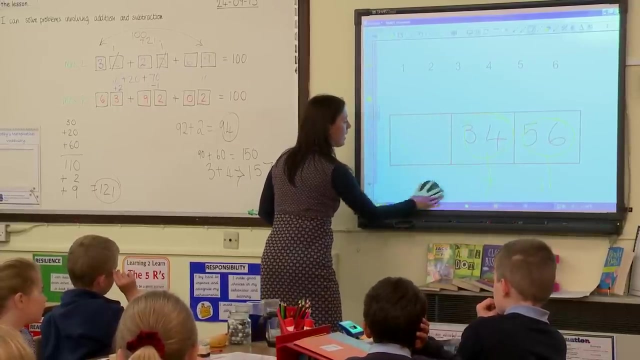 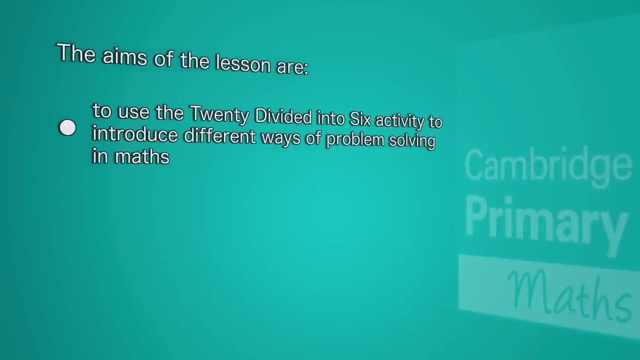 is Seven. Five add six is Eleven. Have I got equal totals in those three boxes? No, No. This allows the class to quickly and confidently familiarise themselves with what they're required to do. The aims of the lesson are to use the 20 divided into 6 activity to introduce different ways. 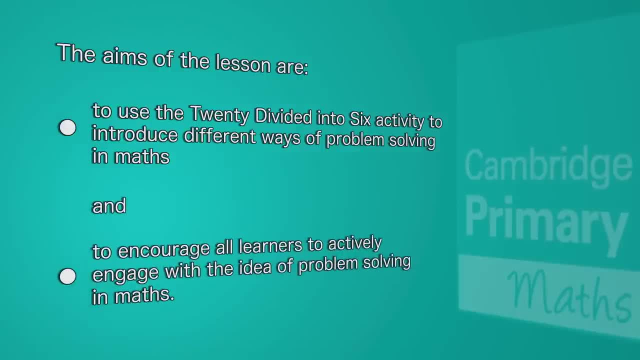 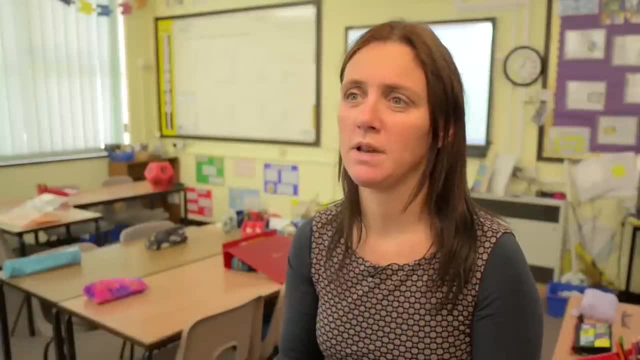 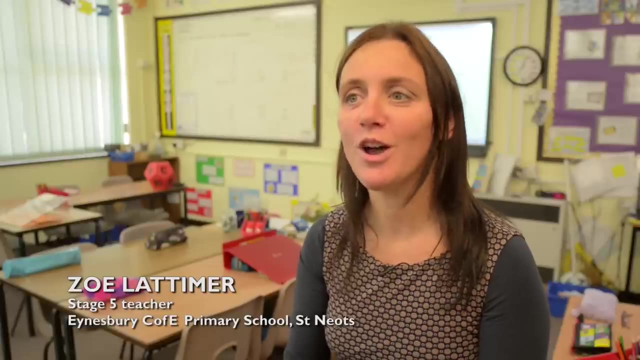 of problem solving in maths and to encourage all learners to actively engage with the idea of problem solving in maths. There's no point planning a lesson as you're responding to where the children are, So you can't plan too far in advance because you might not know where they are in a particular. 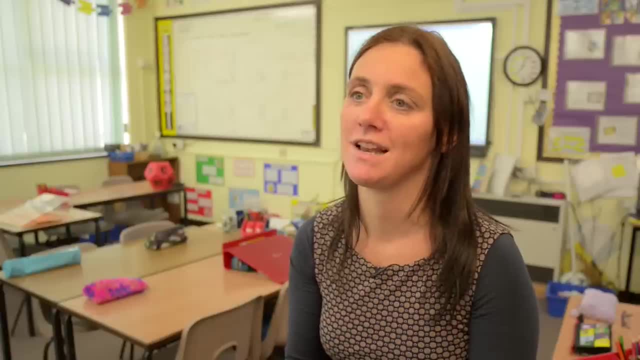 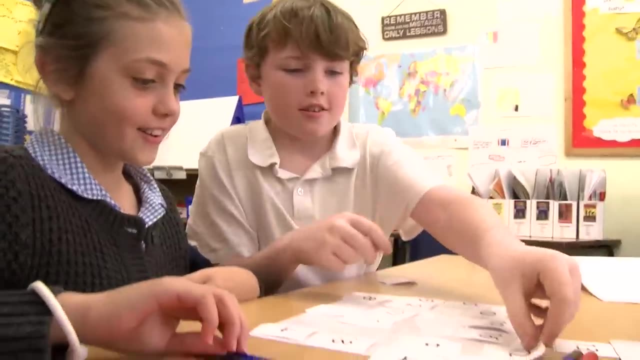 area of maths. So really this activity was planned, having done already lessons in addition and subtraction and being able to get a good grasp on where the children were, As learners take part in the 20 divided into 6 activity. the teacher brings the class together. 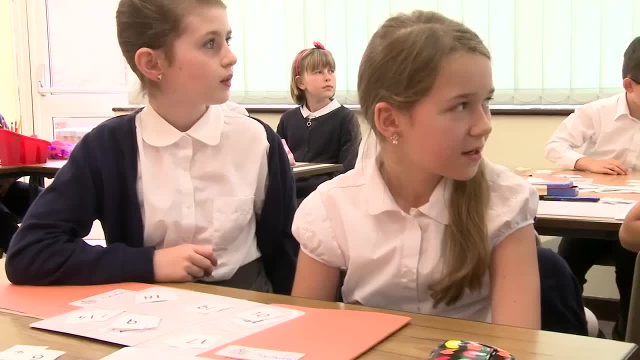 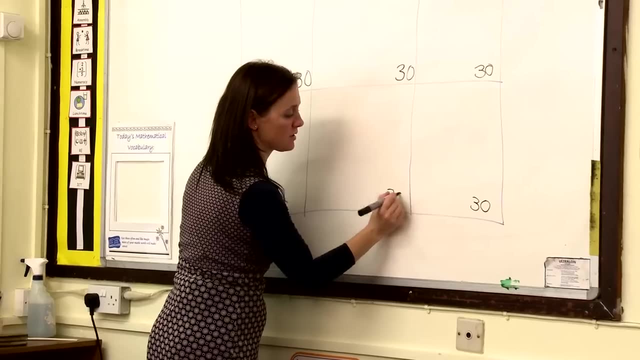 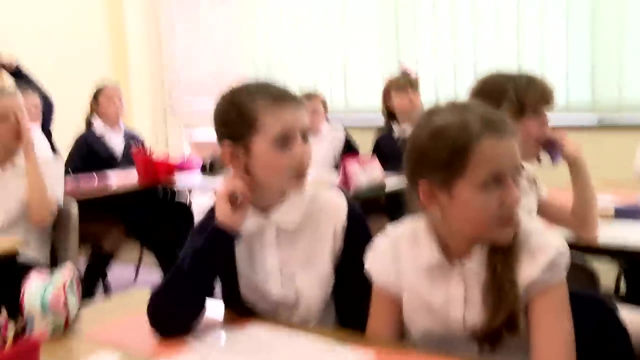 to explore their initial ideas. Camille and Taylor managed to put a total of 30 into each pile. That's great. So we had a total of 30 into each box with different cards. Then she had some numbers left over. Can you remember what were the numbers, or could you? 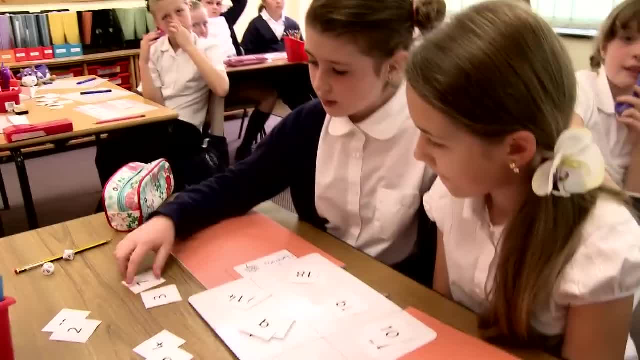 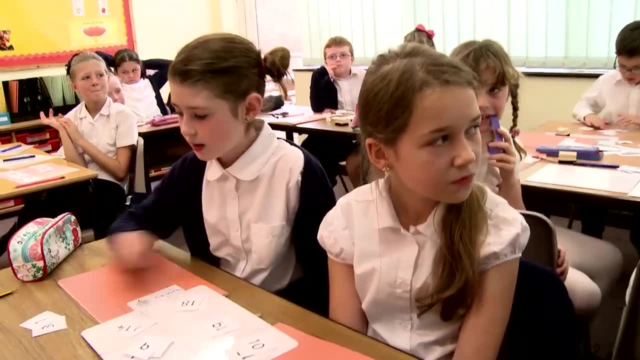 read out for me, Taylor, the numbers that you had left over. We had 3 and 7,, 2 and 8 and 6 and 4.. What can you tell me about those numbers, Taylor? They all added up to 10.. 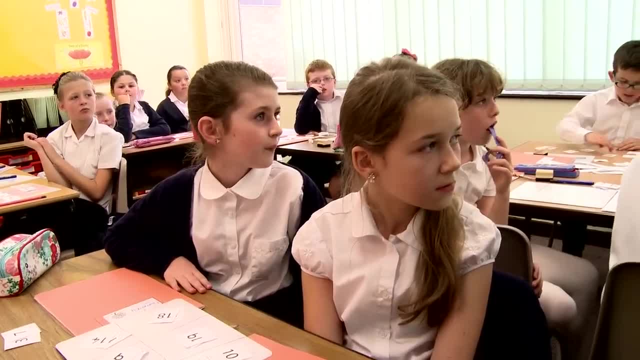 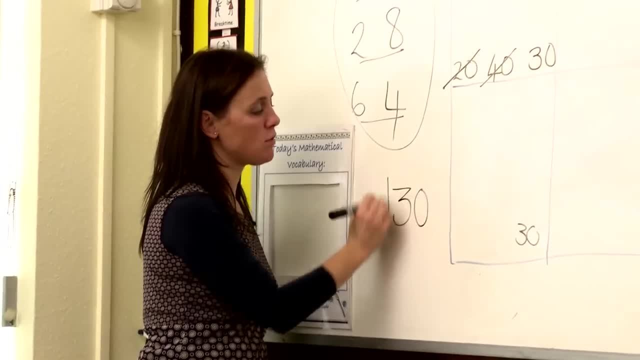 Which in total gave me 10 and 10 and 10 more 10. Which was 30. 30. So we've got 30 more to add in. Camille, you've got 30 more to add in. 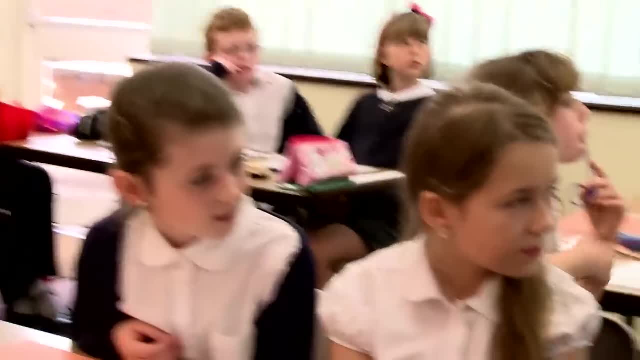 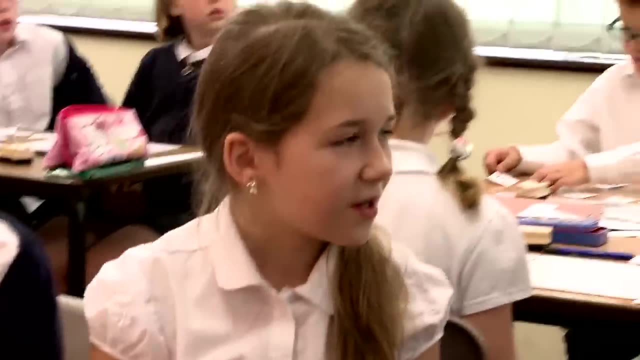 Explain to me what you told me about how you needed to know what went in each box. We needed to add 5 in each box. Why So like to make it 35 in each box? because that's the only way it works. 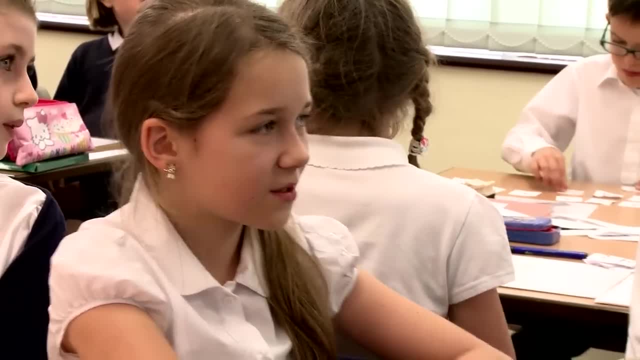 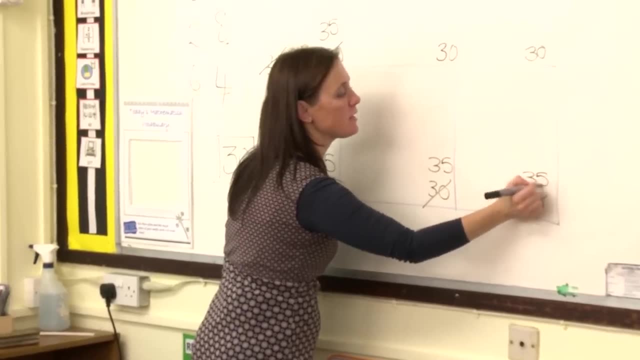 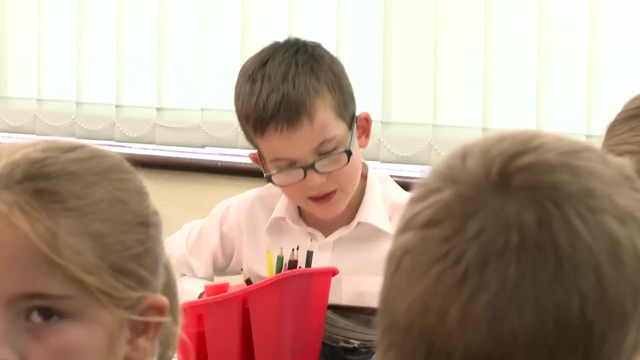 Why? Because that's the only way it works. 35 in each box and you think that that is the total that we are looking for in each box. Another learner chooses a different way to tackle the problem. 1 and 19 is 20,, 2 and 18 is 20,, 3 and 17 is 20,, 4 and 16 is 20,, 5 and 15 is 20,, 6 and. 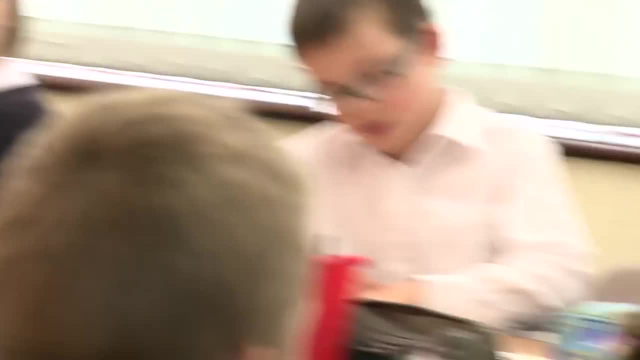 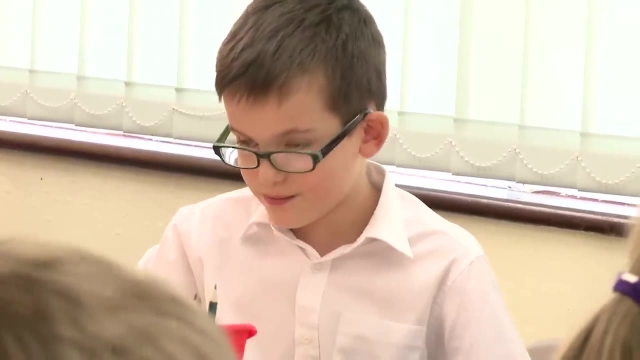 14 is 20,, 7 and 13 is 20,, 8 and 12 is 20,, 9 and 11 is 20.. But two numbers and then 20, and nothing is 20, but the only number we had left was 10.. 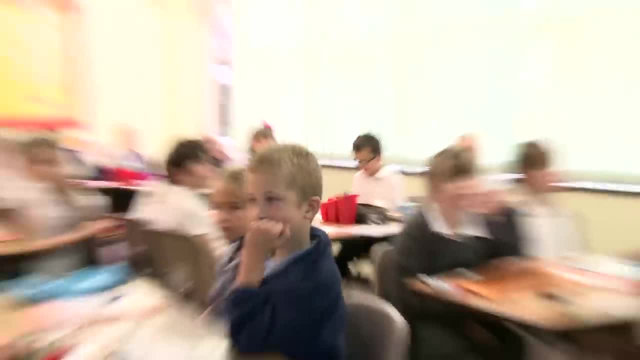 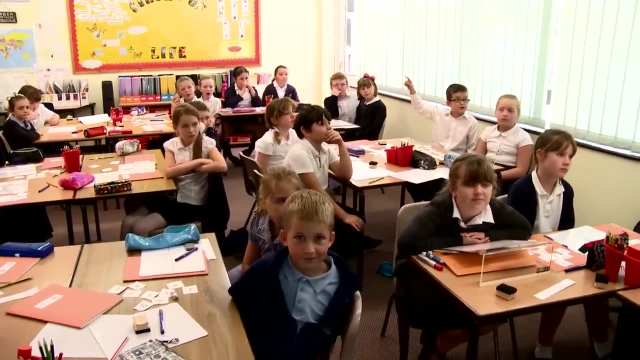 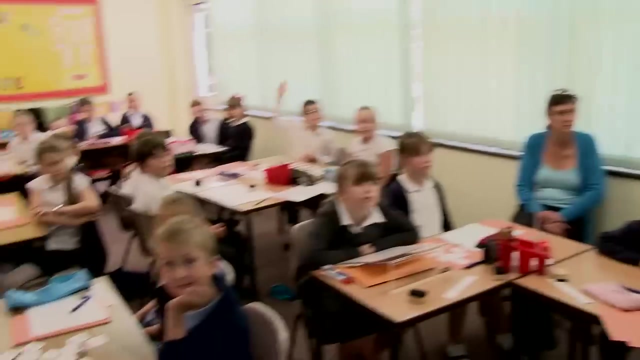 Okay, Hold the 10 and the 20 back. Keep those out of the way. How many groups of 20 have you got? Let's see if Jessie's strategy comes up with the same total that Camille and Taylor: 9, lots of 20,, which gives us a total of 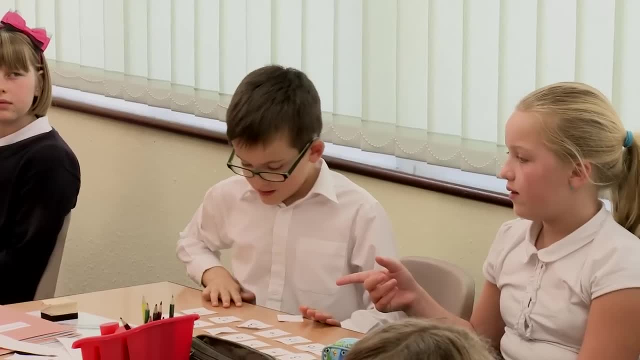 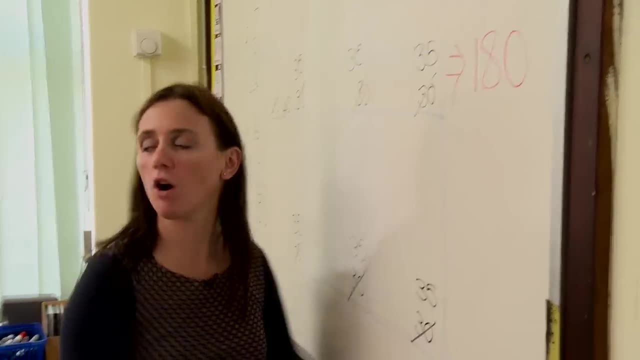 Is that? Come on 9.. 180.. Good boy, 9, 20s are 180.. What have you got left over? Which two-digit cards couldn't you 10 and 20.. Add 10.. That's 210.. 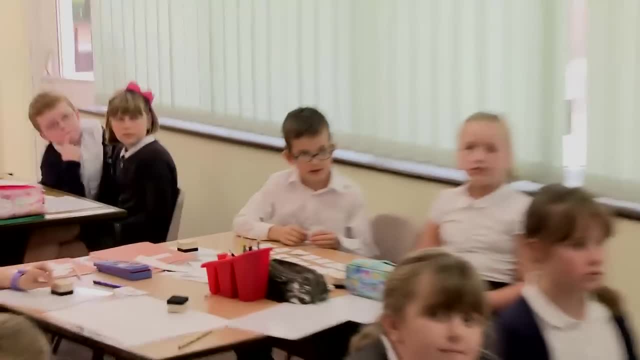 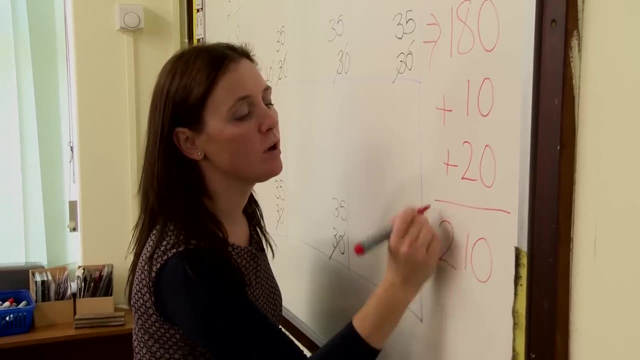 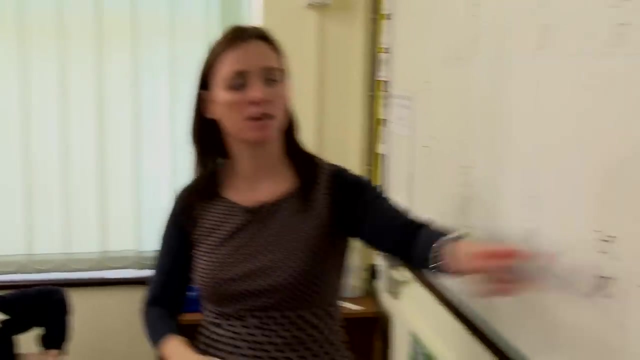 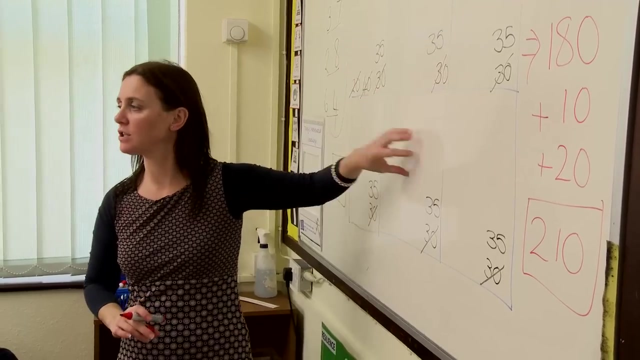 Good boy, 210.. So we know that the total of 1, add 2, add 3,, all the way up to our 20, is going to come to 210.. Yes, I need to split that 210 over 6 boxes. equally. 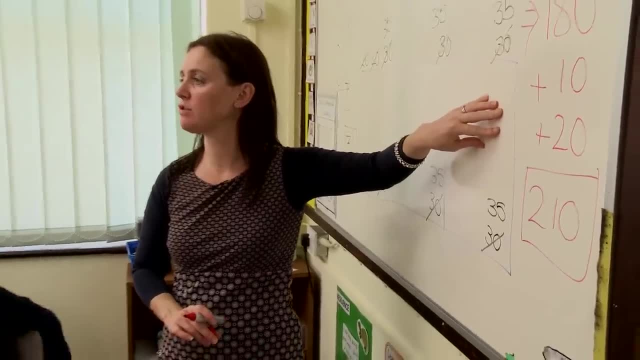 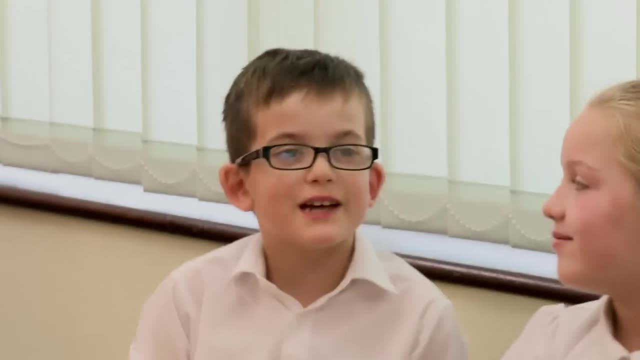 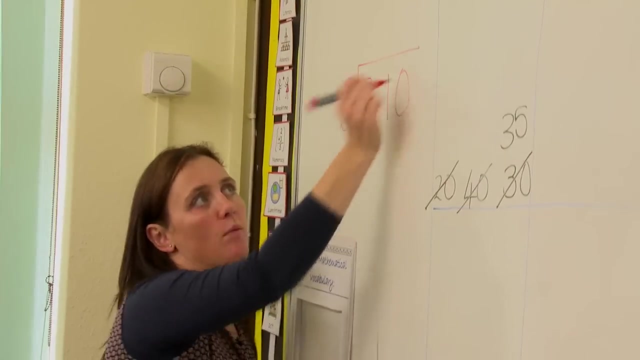 What calculation would I do to split 210 into 6 equal boxes? Jessie, I don't think I can not ask you: 210 divided by 6.. 210 divided by 6. How many 6s in 210? 210. 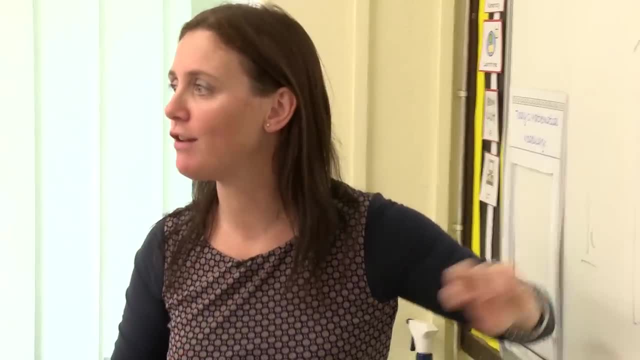 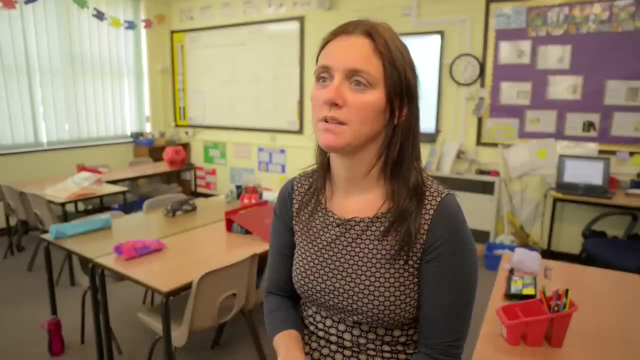 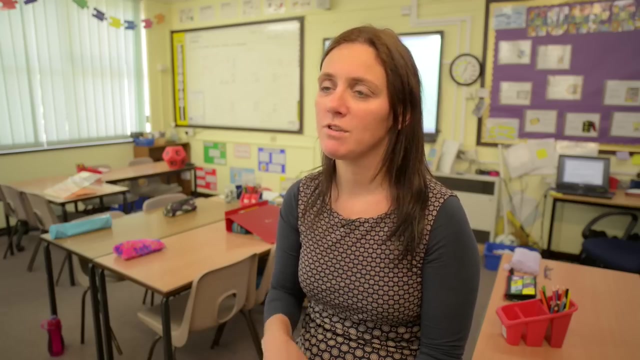 It's an opportunity to share progress and helps the teacher to understand which learners need more guidance. Second method activity is taken from the Enrich website, which is really good for us in school because it encourages children. lots of activities on there for them to really apply their knowledge. 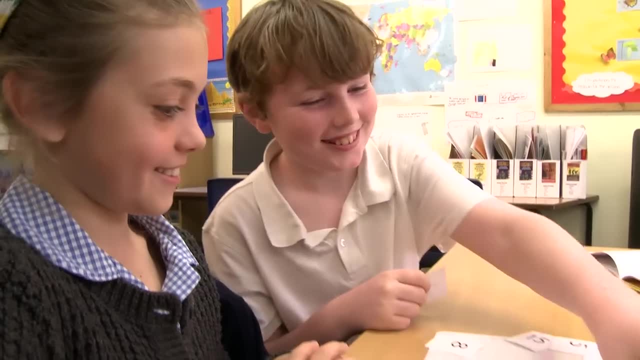 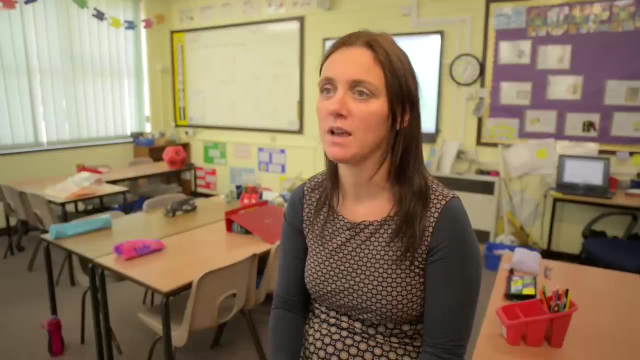 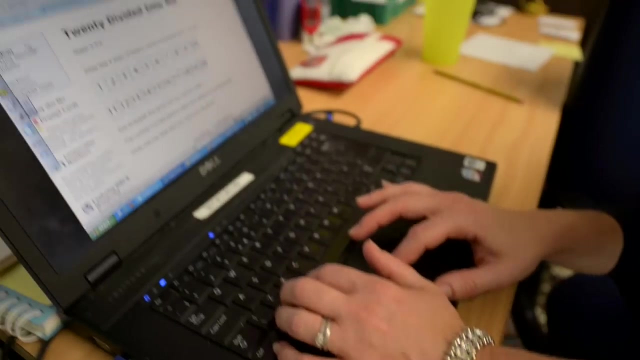 and practice and consolidate skills. So today I chose that activity by really looking to see what would complement the addition and subtraction been doing over the last few days and homed in on the number on the activity, 20 into 6 because that has been mapped for the stage 5 curriculum Once I'd got. 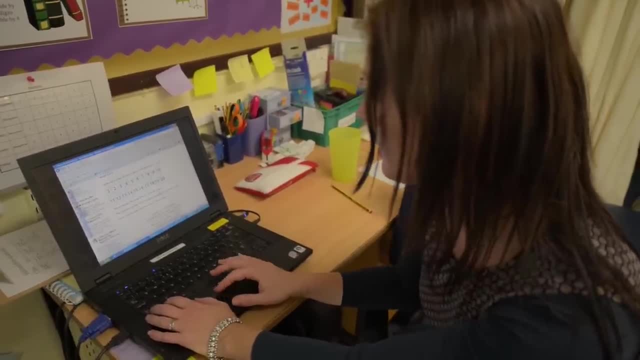 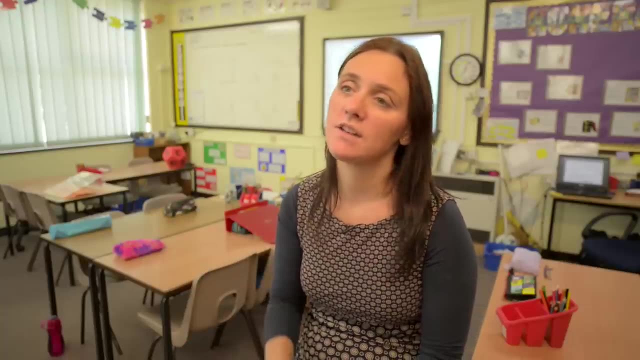 the activity then obviously I had to look at it and see whether or not it was accessible for all the children in my class, and you'd have noticed that they're low ability children. I did obviously have to modify it down slightly so they were just having the numbers 2 to 10 to use for their activity. 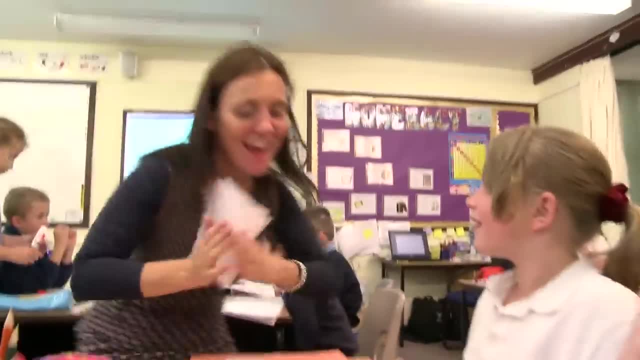 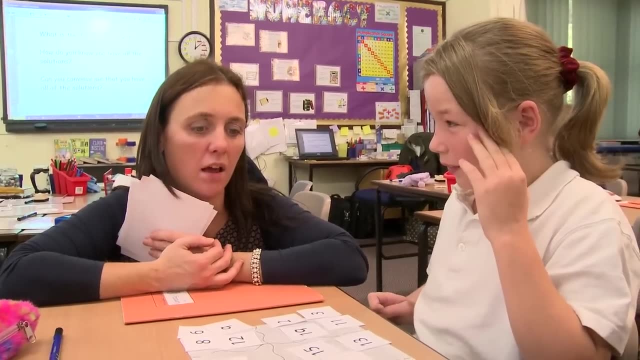 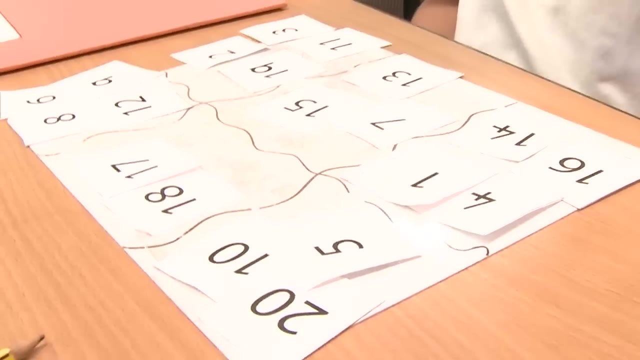 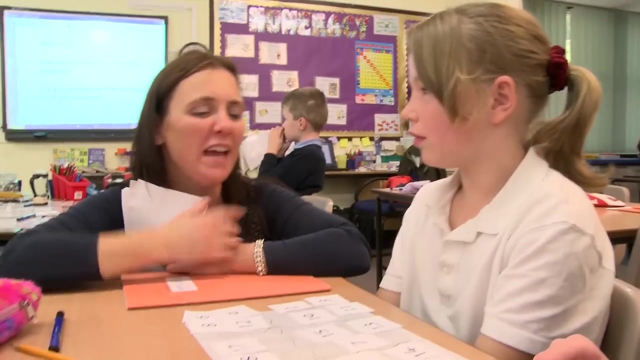 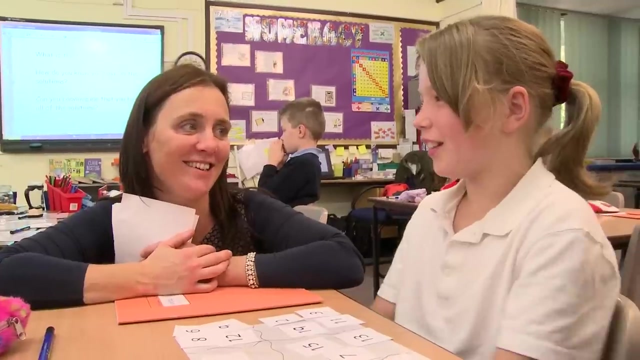 The theme of problem-solving continues and the teacher finds out how another learner solves the problem of 20 divided into 6.. The teacher introduces the idea that there are many ways to solve a problem in maths. Why do you think there's another solution? 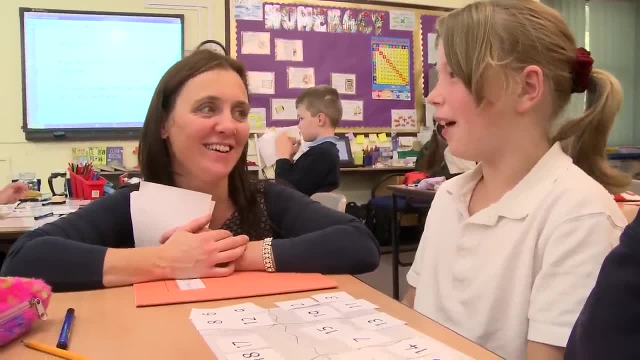 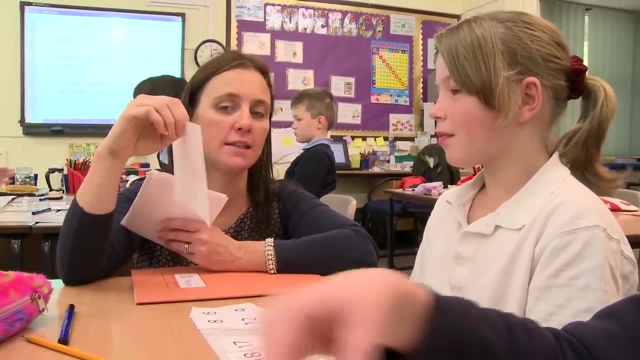 I mean there's another, Because when there's a challenge, there's work to try to get it right. Okay, right, well, I'm going to ask you to record that in your maths book. I'm going to stick this in and then record the way that you've solved it, and then we're 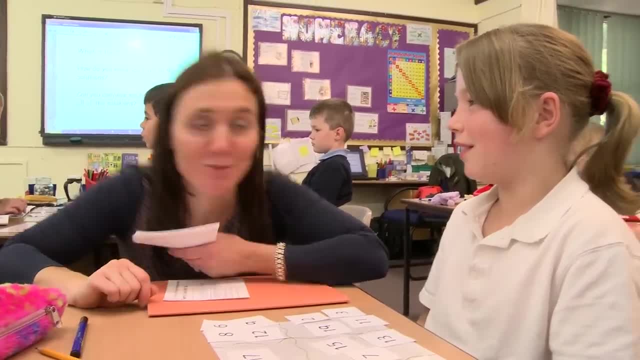 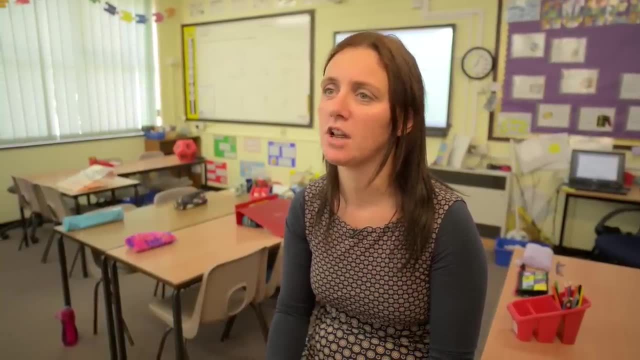 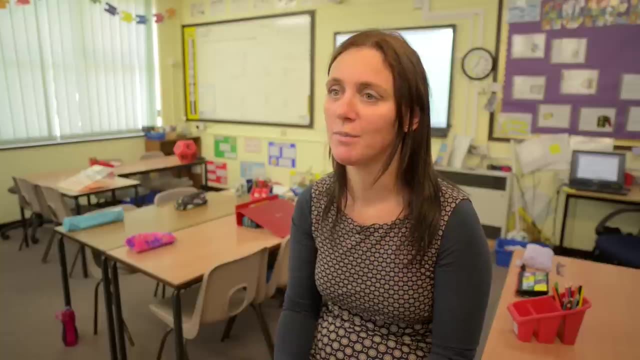 going to have a think about if you've got the only solution, if there's no solution. Problem-solving is really important in maths in terms of encouraging children to start to explain, to generalise, to reason, to justify- All of those higher order thinking skills which obviously go across the curriculum can be really 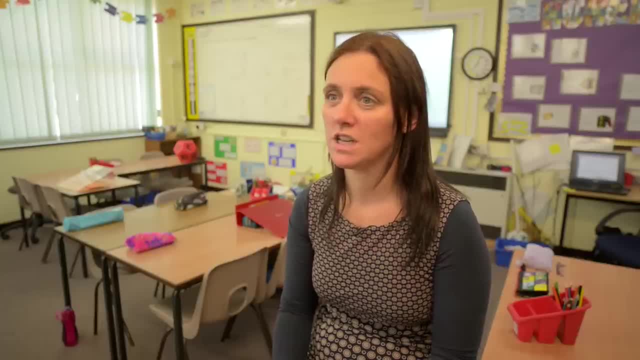 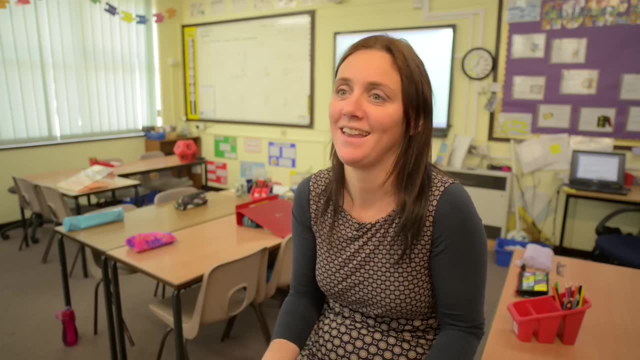 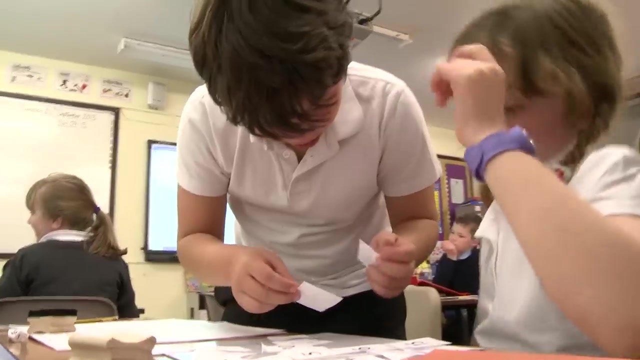 enhanced in maths learning. We do a lot of teaching from a kind of problem-solving angle and it does really benefit the children because it's thinking about. it's the thinking about thinking. Let's add 9.. What does that make 10?? 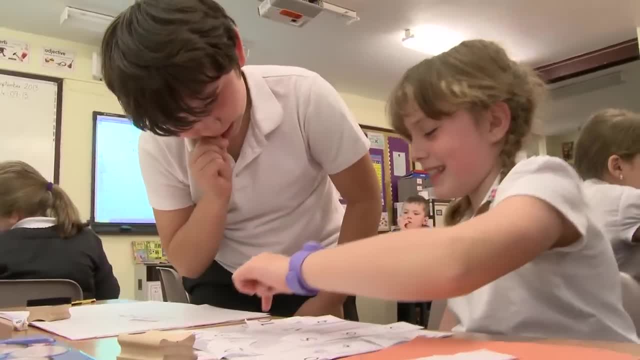 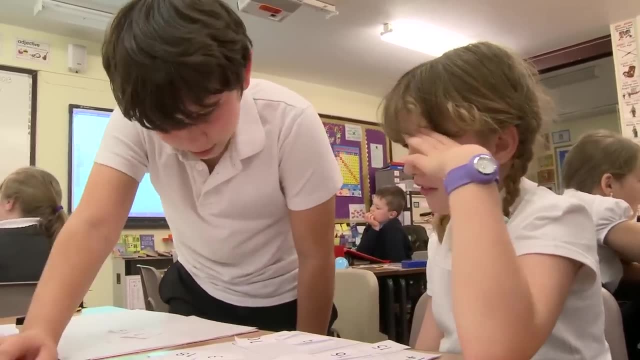 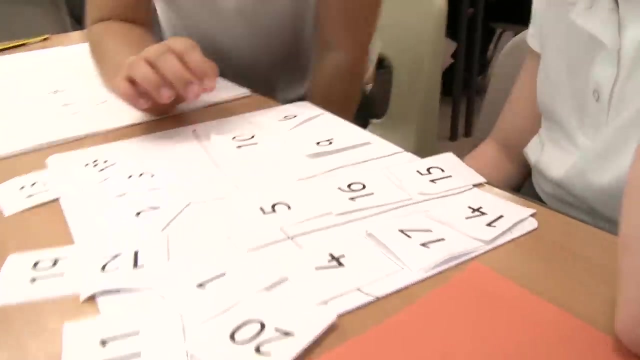 That makes that is 13.. Add 10 is 23.. 23 adds 4 to 10.. Okay, do this one then, because we've already used the 17, so we're only allowed to use 1.. So do 10, add 9, 19.. 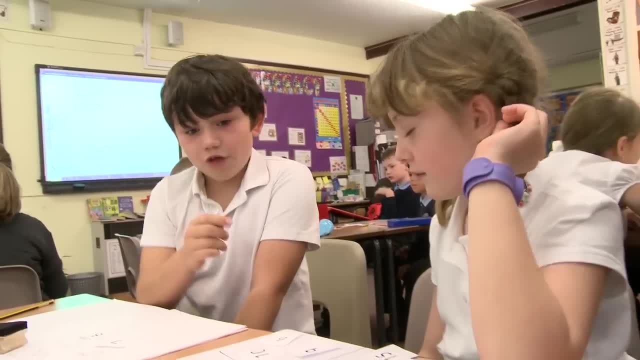 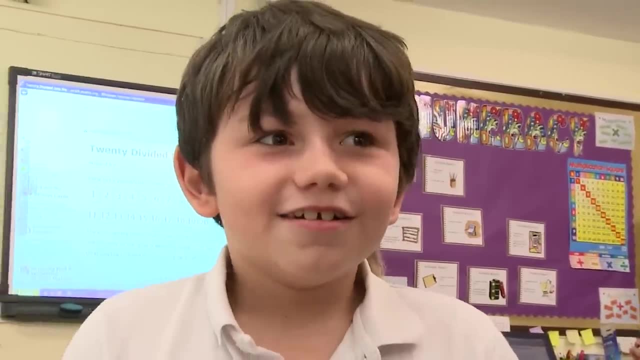 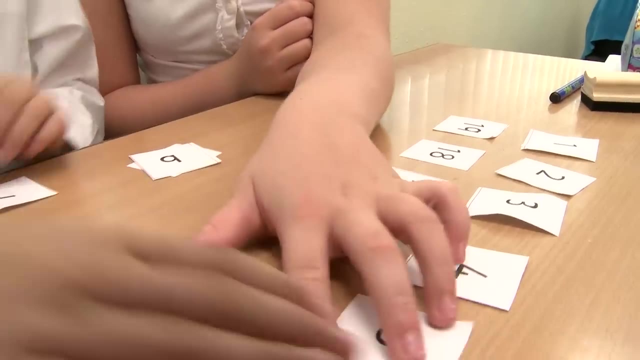 Add 1 because there was 25. 25. Something was like really hard and then when you did it was like yes, I did it, and then it was just It was really challenging, which makes it like really like good. The teacher evaluates the lesson and shows how the activity can be used to judge the. 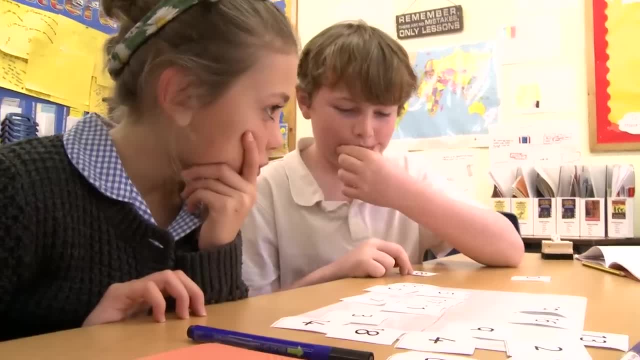 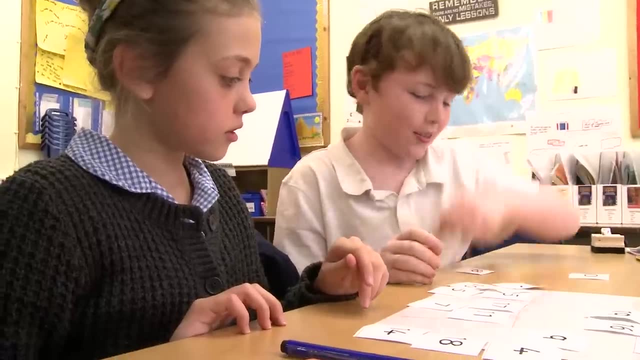 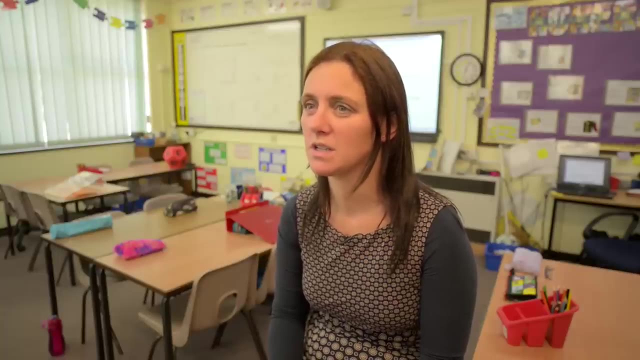 progress of individual learners and how learners can build confidence in mathematics by working together. I think the dialogue that goes on between the children is really important. If a child is encouraged to explain their thinking, then actually they start to internalise it and really get to grips with the understanding. 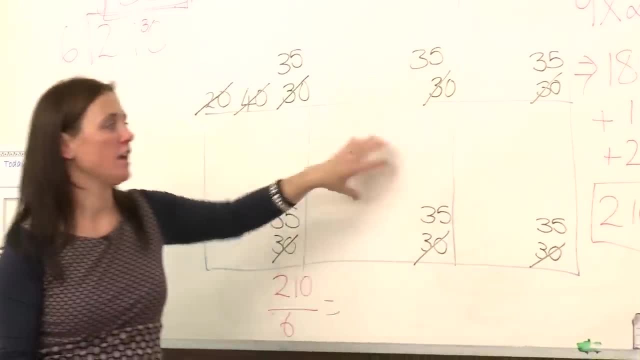 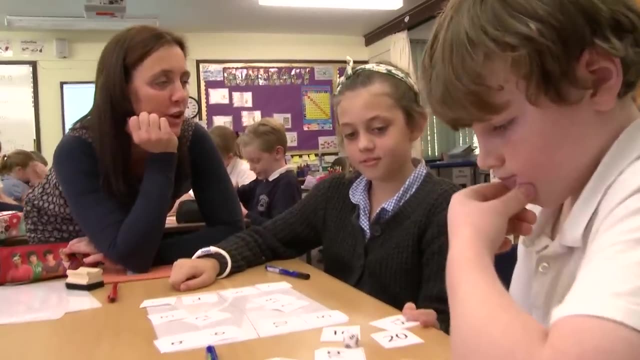 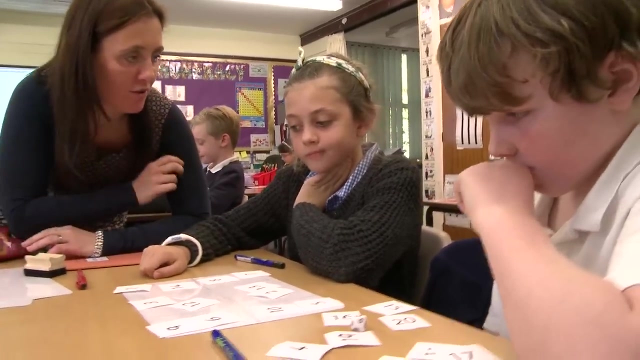 We do a lot of explanation, discussion, paired work, and that seems to benefit both the higher and lower retainers. Are you going to be able to build up to 20 with the numbers you've got left over? No, So could you revise the first 20 you've decided on? 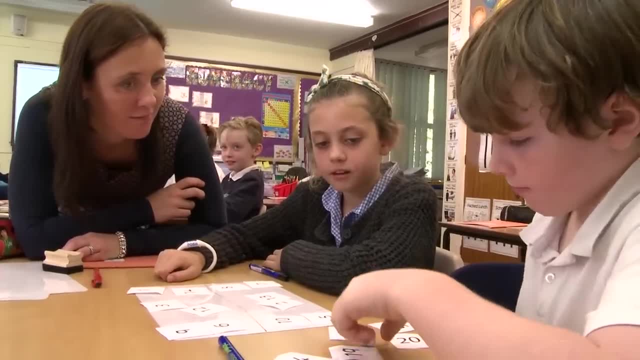 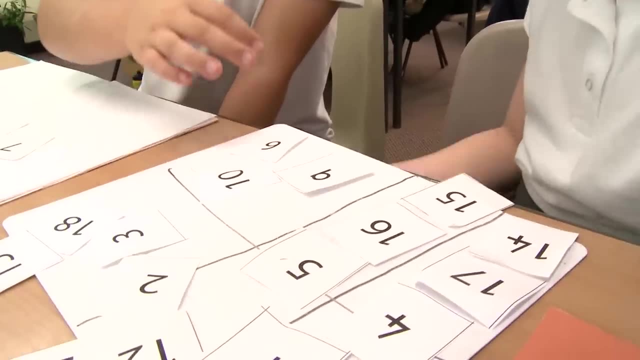 Go on then, Right? so yeah, We need to take all these off. We need to make 20 and 1 the same 25. 25. And what is this? That's 32. 32. So what was that again?